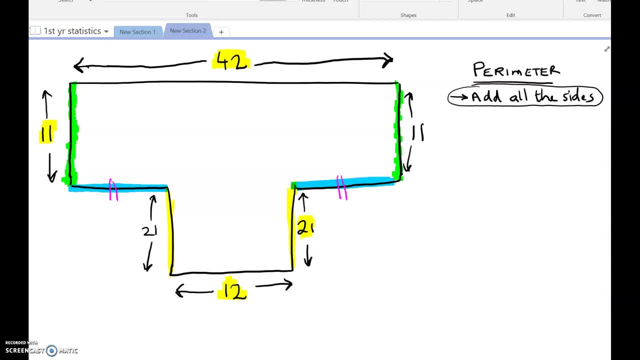 Now, how can we get it? Well, just like the other questions we did yesterday, if you look up along here, all of this is 42. All of it. So all of this here would also be 42. Now, we don't want all of this here because we're missing a bit, aren't we? We only want what it is from here, and then from here to here, These two bits. 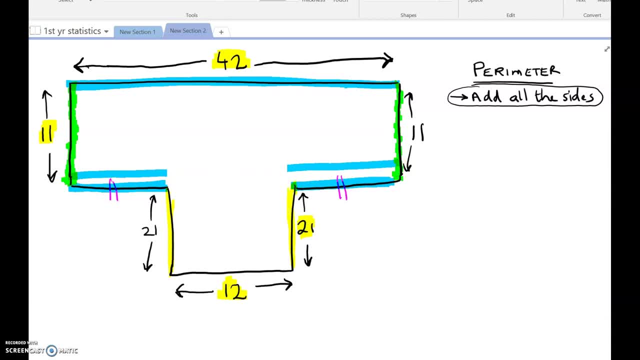 Now we know all of it is 42, but we want to remove- okay, take away- this bit because it's not part of it And we actually know how long this bit is. We know how long it is from there to there: It's 12.. See the way it's 12 here. That means it's 12 here. 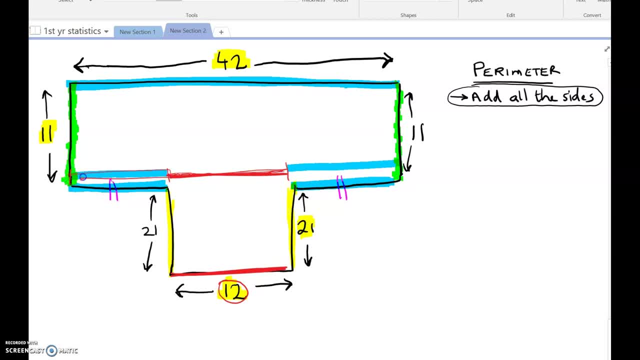 So these two bits must be 42 without 42. So if we get our 42, and we take away the 12, we're left with 30. That means that when you add this and this together, these two bits here, this and this together, it adds up to 30. 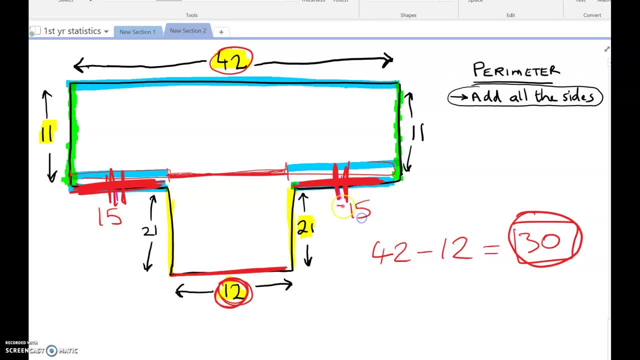 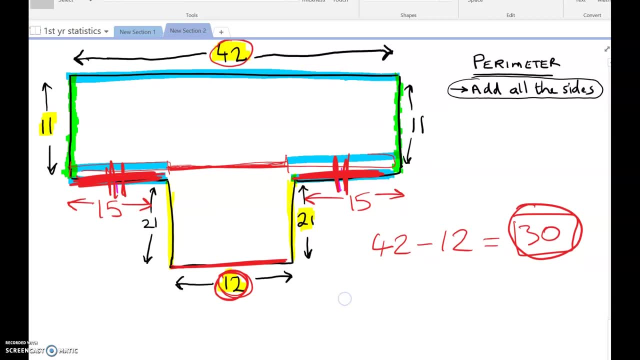 So that must mean there are 15 each, because 15 and 15 is 30.. Now we can get the perimeter. Okay, Remember to get the perimeter. you can add all the sides together. So we have to go through it very, very slowly. We'll start up here: 42 plus 11.. I always circle them when I'm doing them so that I don't forget that I've done them. 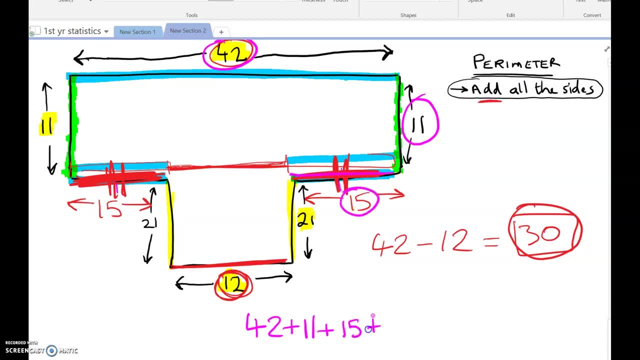 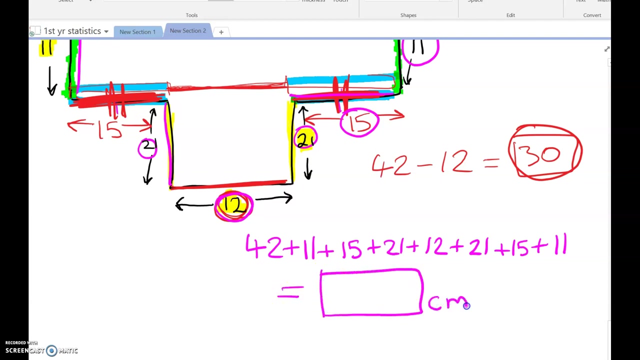 15,, 21,, 12, 21,, 15. And 11. Type it all into the calculator And whatever you get is the answer. You don't say centimeter squared, because it's not area, it's just perimeter. Okay.